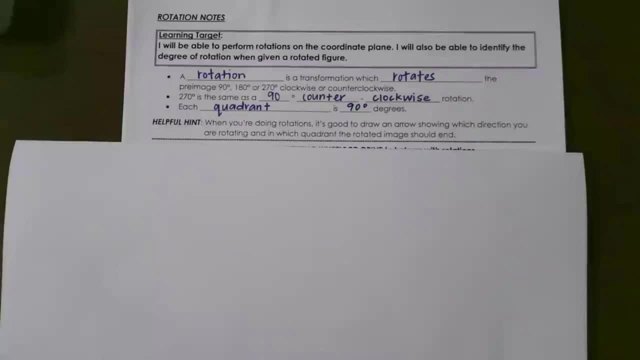 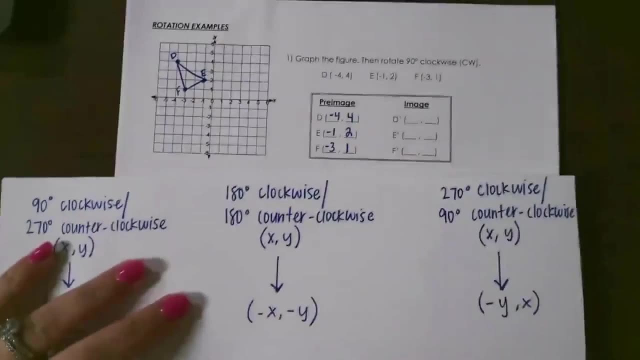 rotations. it's good to draw an arrow showing which directions you are rotating and which quadrant the rotated image should end. Let's look at some examples. So this first one: we want to graph the figure and then rotate it 90 degrees clockwise. So 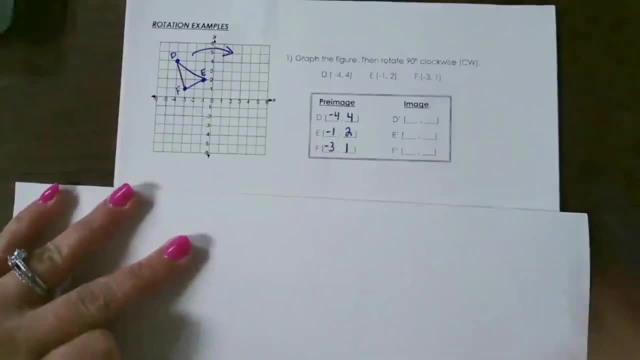 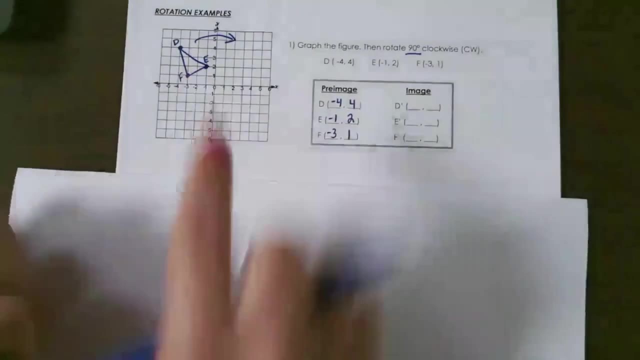 clockwise is going to be this way, and 90 degrees is only one rotation. Okay, so our pre-image, these are our points, and I went ahead and plotted those on the graph. So the easiest way to do this is to draw an arrow showing which directions you are rotating and which quadrant the 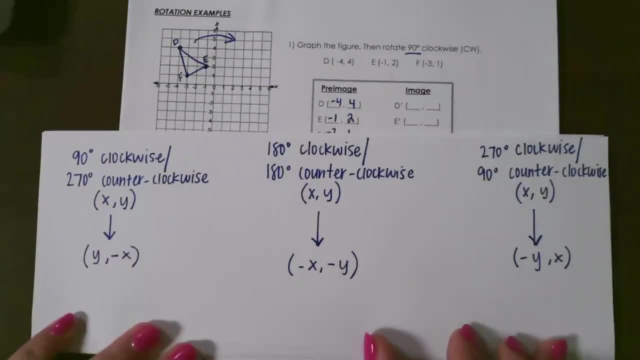 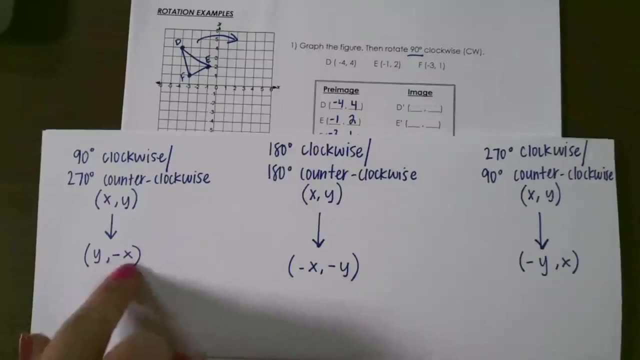 rotated image should end. The easiest way to do this is just to memorize each of these different rotations. So again, this time we're doing 90 degrees clockwise, which is going to take our x and y to y negative x. So that means our y value becomes our x value for each of them. 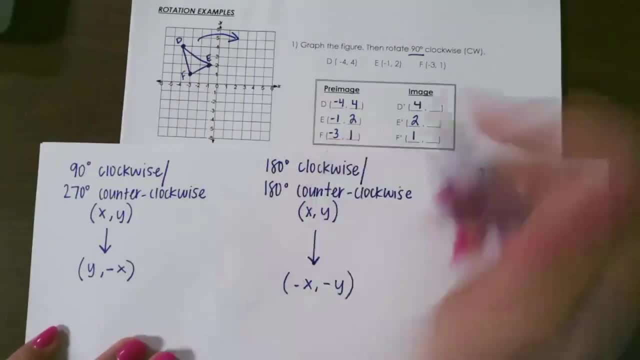 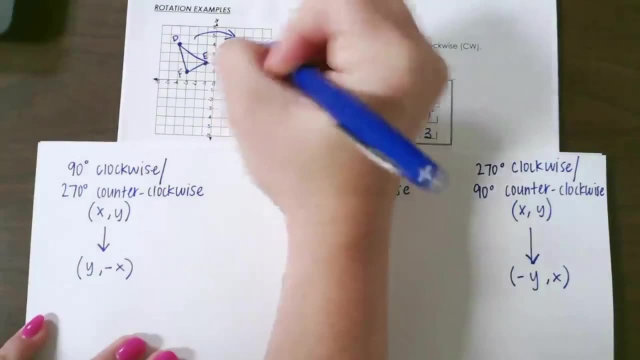 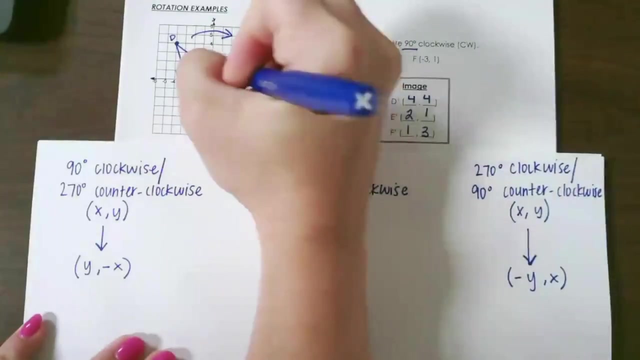 and then this is going to become a negative version. Since it's already negative, it will become positive. So then we plot those points. So I have 4, 4, which will be d prime, 2, 1, which will be e prime, and 1, 3,, which will be f prime. 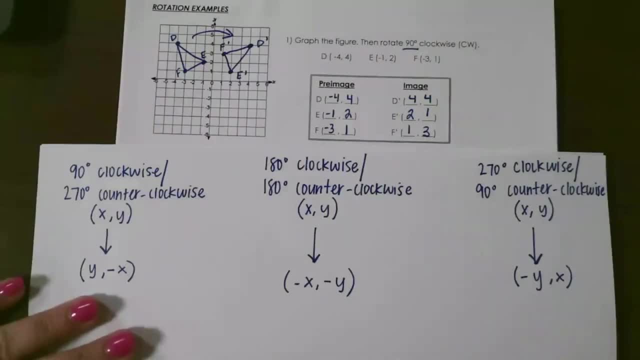 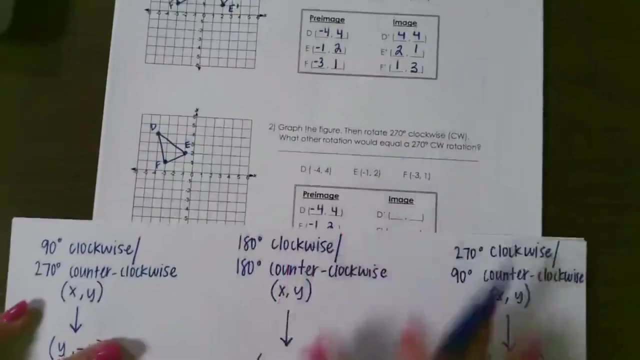 So that shows a 90-degree rotation clockwise on our graph. So next let's look at the next one Graph, the figure, then rotate it 270 degrees clockwise. So here's 270 degrees clockwise and it shows us that x is going to be y and y is going to be y and y is going to be y. So 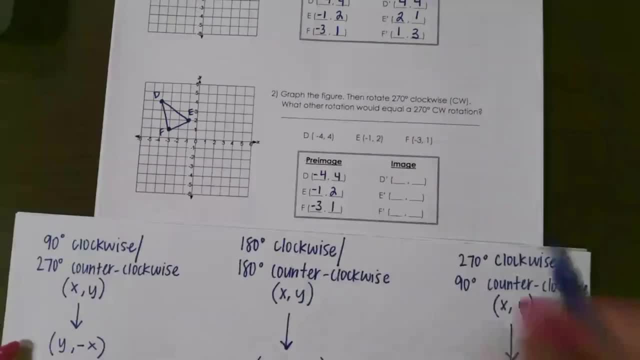 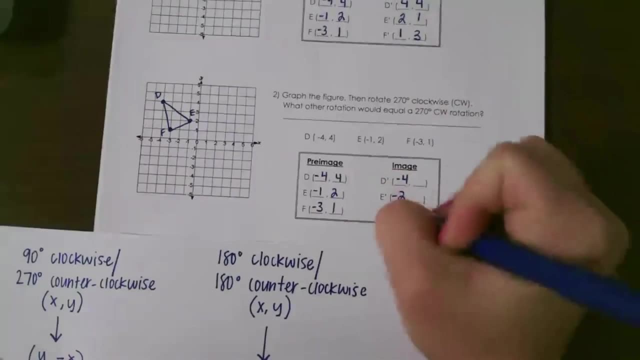 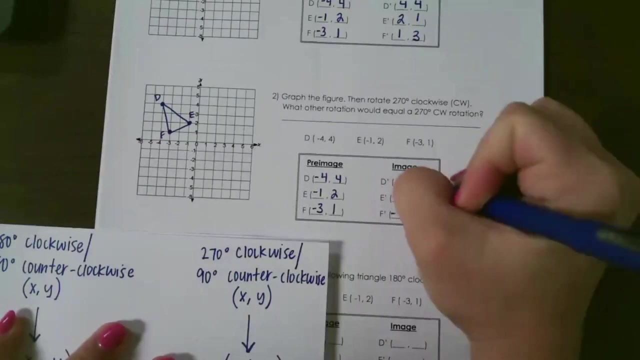 y becomes negative y. positive x, So negative y. so that would be negative 4, negative 2, and negative 1, and it's going to become the same x. So we don't change anything about x. So this one's negative 4, negative 1, and negative 3.. And then we just plot those points. 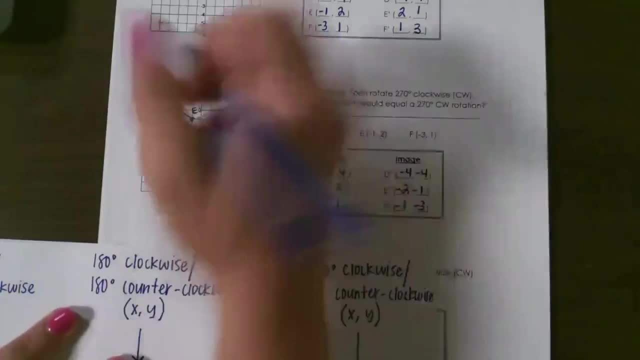 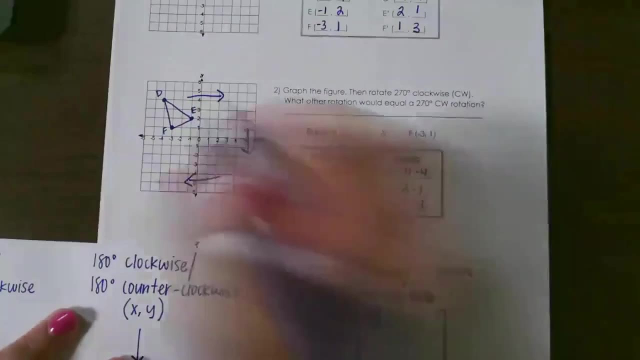 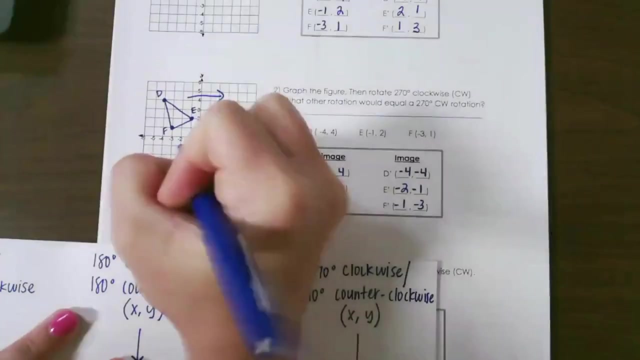 on our graph. So 270 degrees clockwise is going to be 1,, 2, 3.. So it should end up over there. Negative 4, negative 4 would be here and that's going to be d prime. Negative 2, negative 1 is e prime.